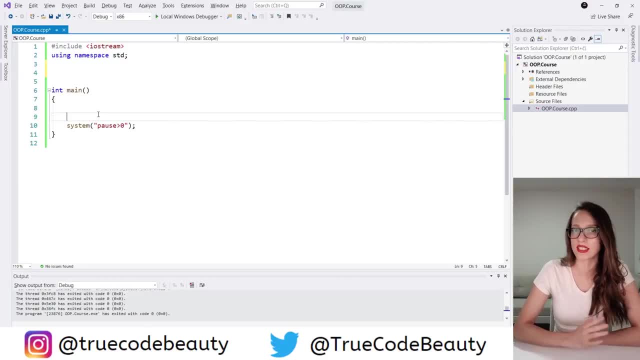 objects. So let me explain the difference: What is a class and then what is an object? A class is going to represent a template, meaning a blueprint, and then an object really represents an example of that class, an instance of that class, For example. 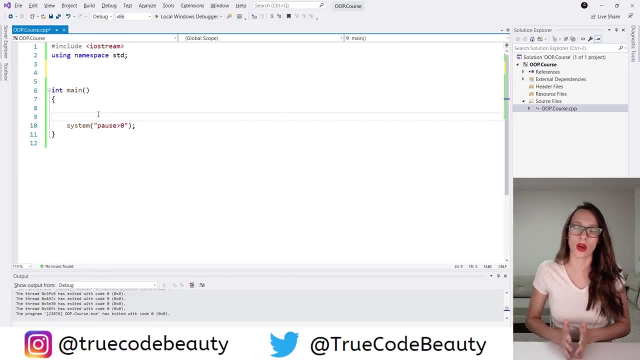 a class can be a fruit, and then an object of that fruit class can be an apple, a banana, a peach, Or another example: a class can be a car, and then an object of that class can be a Volvo, a Ford, a BMW and so on, And that car class, for example, has some. 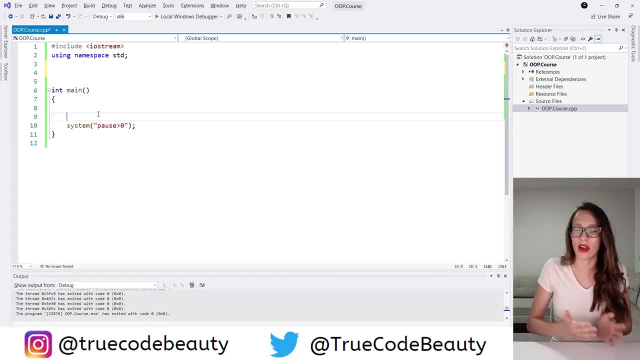 attributes that are going to represent an object. So let me explain the difference. We have attributes, and then it has some behaviors as well. Now, what are attributes of car class? Well, a car has a name, for example. That's an example of one attribute, And then it has a price. 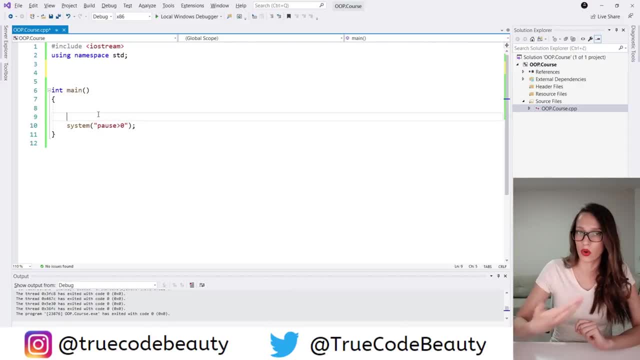 and max speed and color and so on. And then behaviors of a car can be: drive, for example, and then brake as well, and then change color, and so on. So here we are going to create an example of a class, and then we are going to create an example of a class. And then we are going to create 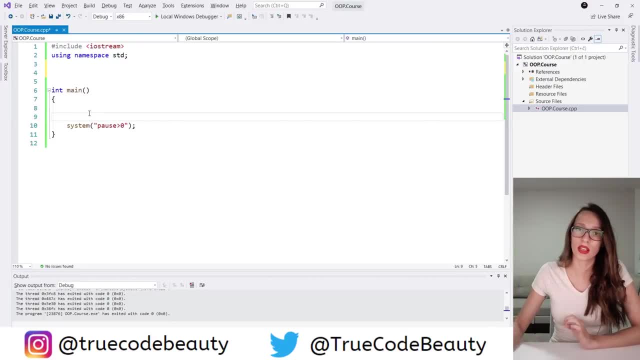 are going to create an object of that class. so the class that i want to create is going to be called youtube channel. so in order to create a class, you write class and then you give a name to your class. so here i'm going to say youtube channel, like this, and then you put these curly. 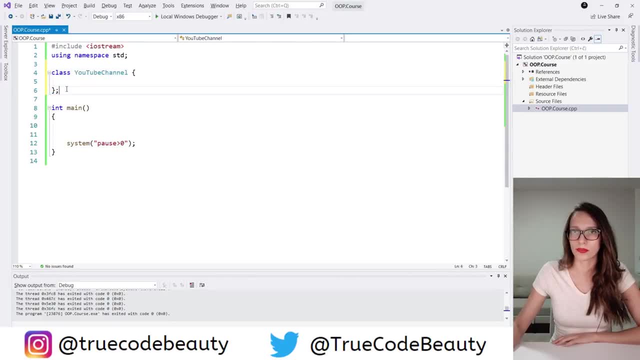 brackets, and at the end you will have to put a semicolon. and now, here you will put the members of this class. now, one thing that i haven't mentioned is that class is user defined data type. we have already talked about data types in this course or in c plus plus for beginners course, so 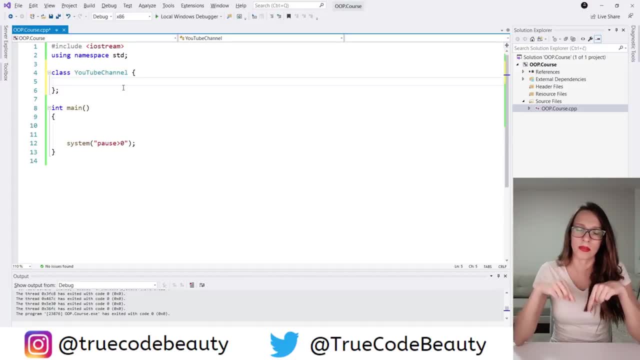 if you haven't watched that, make sure to do so. i'm going to link it in the description and then here as well. so we have talked about basic data types such as integer, floating point number and then boolean character, double string. but a class is going to be a user defined data type which is going to allow you to represent. 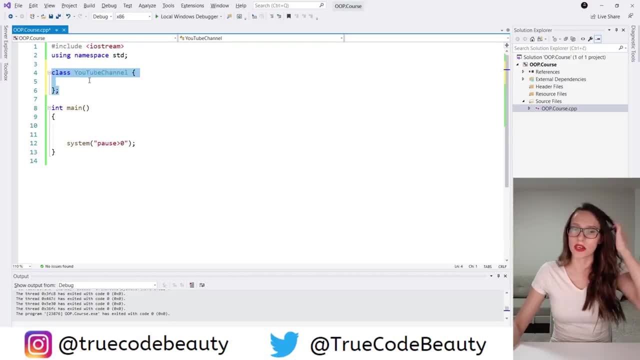 a real life object in programming and in this particular situation, i want to represent a youtube channel. so let's think of attributes of a youtube channel. what is something that describes a youtube channel? let's say, for example, that each youtube channel has a name. so that is going to be a string. 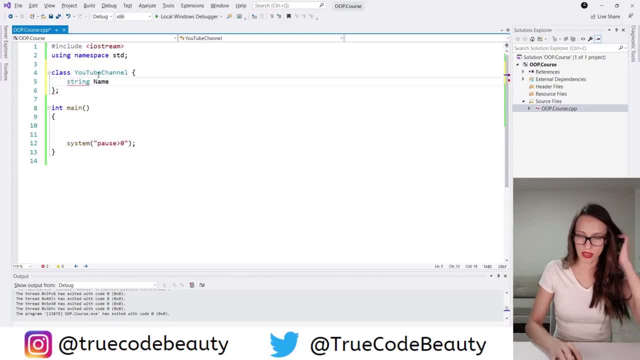 variable. let's say string name, like this. so these attributes are going to be represented with variables. so one of the attributes is going to be name, and then let's say another is going to be string owner, owner name, like this. and then let's think of another attribute. let's say that: 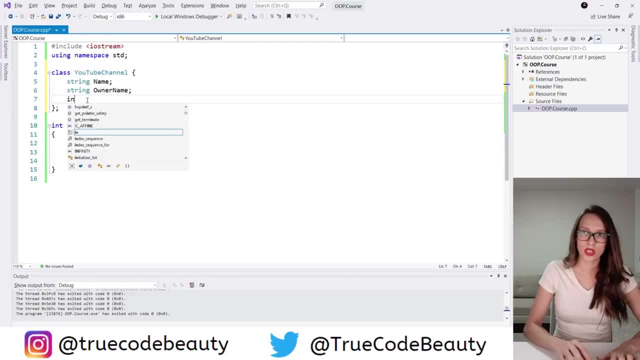 each youtube channel has a subscribers count, so int subscribers count like this. and then let's as well create a list of published videos. so i'm going to say list and let's call it published video titles. so that is going to be type string and it is going to be 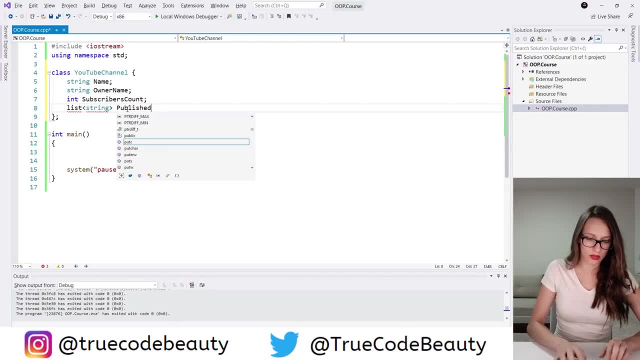 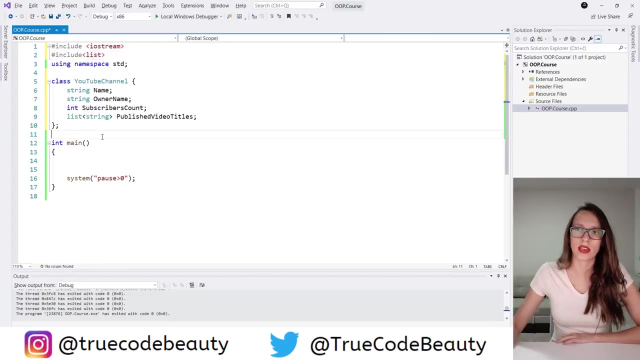 called published like this. now here it says that this list cannot be used because we haven't included um it here. so here i'm going to say attribute list and now this should be accessible. okay, now we don't have that error anymore, and what I want to do here is I want to represent a youtube channel that has four attributes. it has 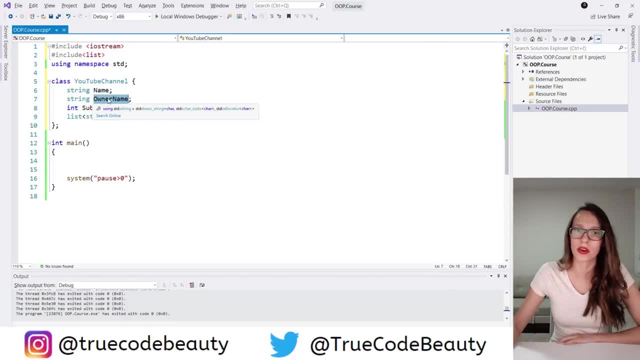 a name, then owner name- you can use email here or whatever- and then it has subscribers count and published video titles. now here you can use another class. here you can say, for example, list of videos. you can create another class that is called video And then in that video class you can put all the attributes that describe a video. 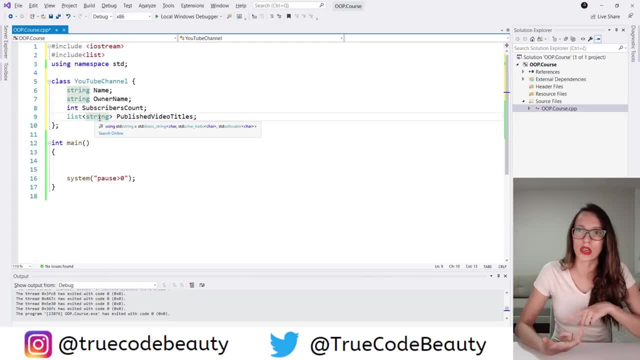 So that can be, for example, a title and then a description: number of likes, number of comments, number of views, the duration of that video, the video itself, you know. But for the simplicity of this particular example, I'm going to use just the title of those videos. 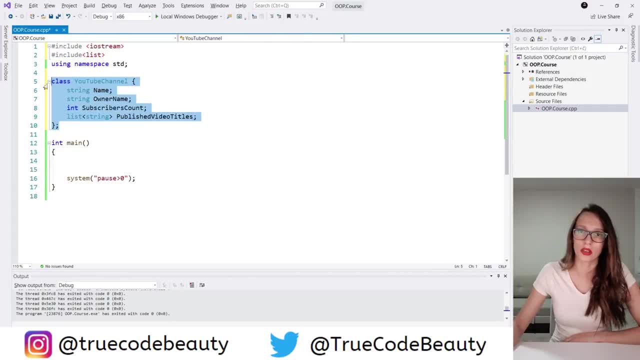 So now, after I have created this YouTube channel class, what I can do is I can create an object of that class. So let's say here that I'm going to create an object. So how you do that? you say the type, So you put the name of your class, which is YouTube channel, and then you give a name to that variable. 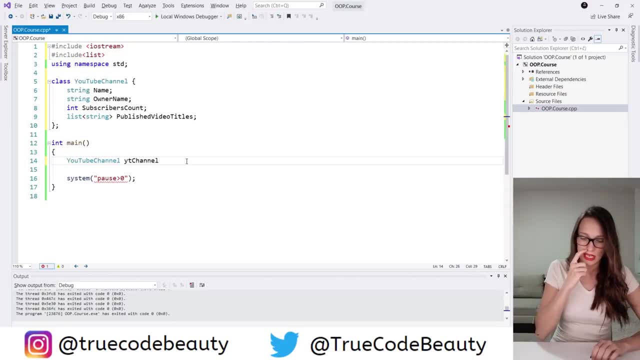 Let's call it YouTube channel, like this. OK, now what I want to do is: I want to, I want to assign values to these properties of my YouTube channel. And how do I do that? Well, you say YouTube channel and then you put dot. 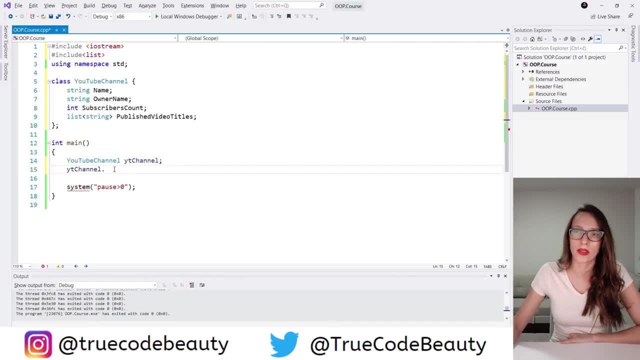 And here is nothing available. but it should be. These properties should be available. when you say YouTube channel, dot, Now why these are not available? It is because all the members of your class are, by default, private And that means that these members, because they are private, 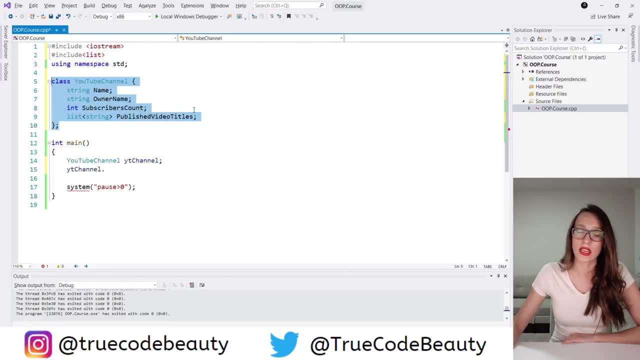 they are going to be accessible only within this class here, And in order to make them public, in order to make them accessible outside of this class, you put public access modifier. So you say here, public, OK, like this: Now this public is an access modifier and it is going to make all of these members. 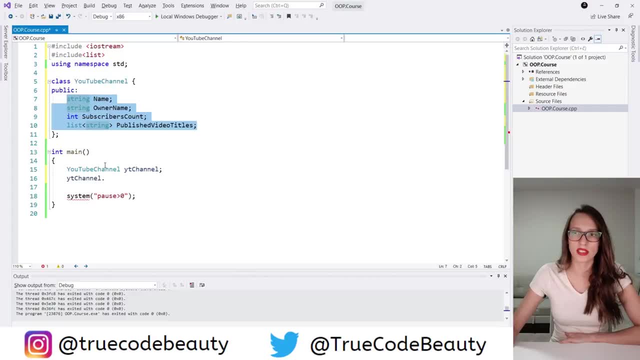 of your class accessible outside of your class, which means that now if I press dot here, you can see name, owner name, published video titles and then subscribers count is available for me now. So I'm going to say that the name of my YouTube channel is going to be: 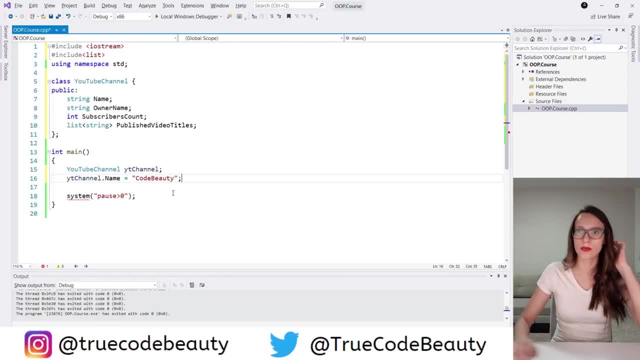 for example, Code Beauty, like this, and then owner name. Let's copy this a couple more times. So owner name is going to be my name, So Saldina, like this, and then subscribers count. Well, let's say this is an integer variable, so we don't need the quotation marks. 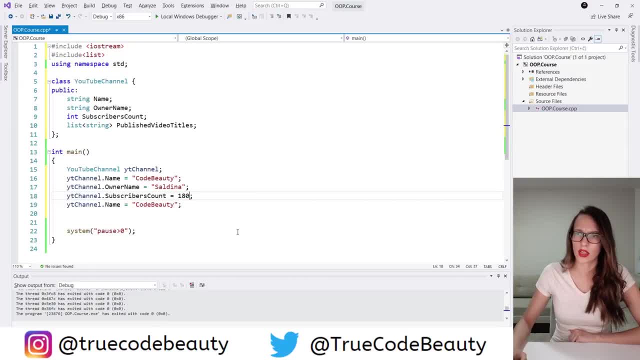 Let's say one thousand and eight hundred people, and then these published video titles. So let's add value to my published video titles list. So here I want to say that I have published, for example, C++ for beginners. Oh, let's say video one. 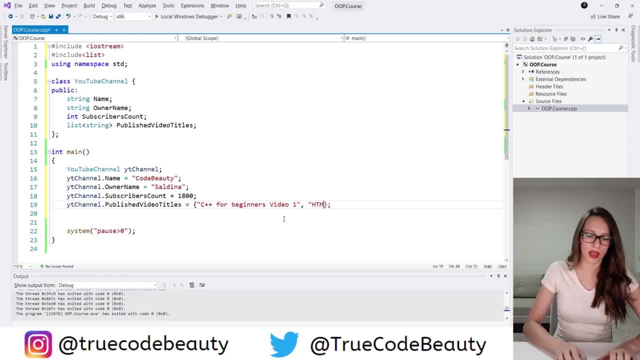 OK. and then let's say HTML and CSS video one. OK, and let's add as well this video. So let's say C++ OOP video one: OK. now, after I have assigned value to these properties, what I can do is I can write out these properties. 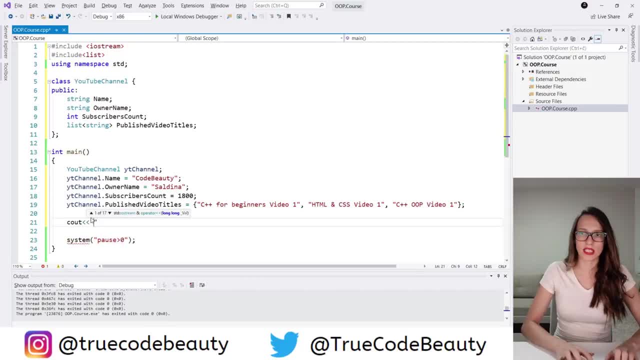 So I can say here, for example, see out. and then let's say name And let's write out the name of my YouTube channel, like this, And I'm going to add an end line and I'm going to copy this couple more times, like this: 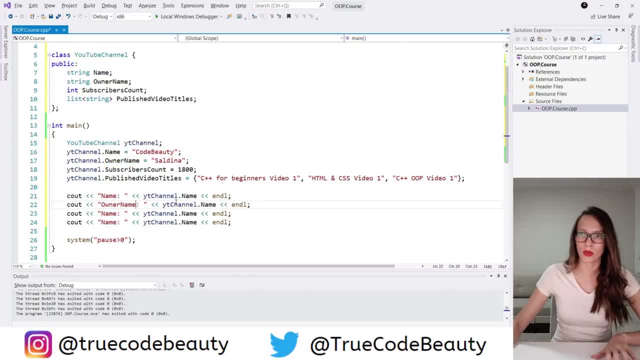 So here I want to write out owner name. So let's put YouTube channel dot owner name. And then here I want to write out the subscribers count. So YouTube channel dot subscribers count. and then published video titles. Now this property- here published video titles- is not a simple property. 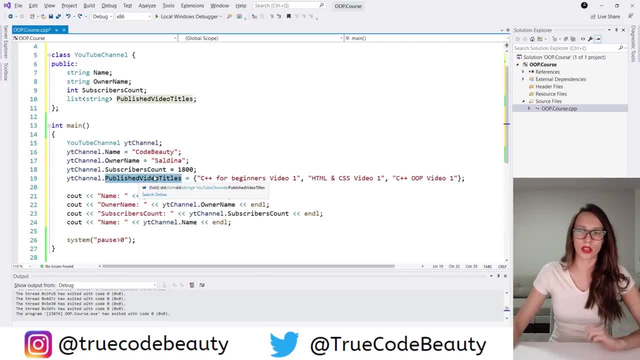 meaning this property here is a list, And in order to write out a list, we are going to use a loop, So I'm going to delete this. And then here I want to create a loop And let's say that we will be using for each loop. 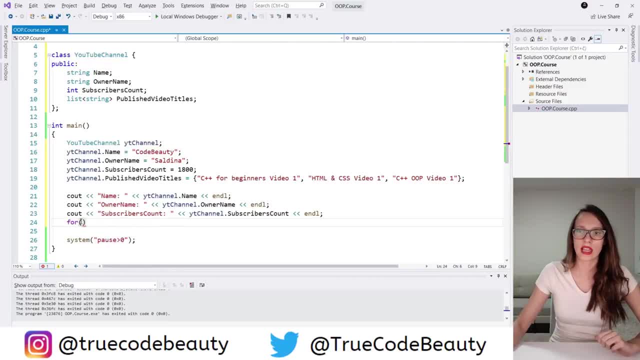 So I'm going to say for, like this, And then here I'm going to write out the type of the value that I'm going to use in my list. So I'm going to say string, because this published video title is of type string. 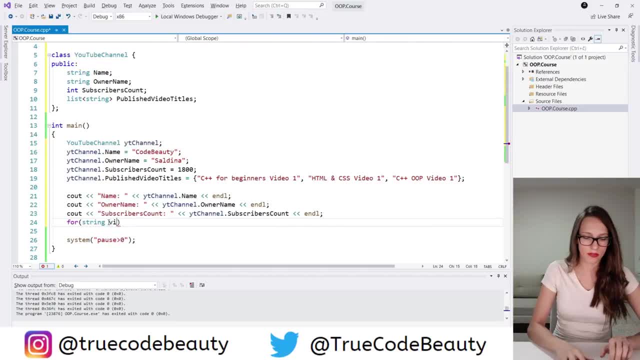 And then here I want to give it a name, So I'm going to say video title like this, And then I'm going to specify the list that I want to iterate And that list is going to be this one here. So it is going to be a list of published videos in my YouTube channel. object: 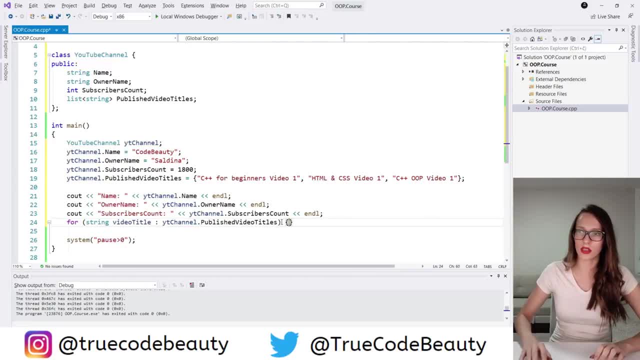 OK, and now in these curly brackets, I'm going to specify the block of code that is going to be executed in each iteration. So what I want to do with this video title is: I want to write it out. So I'm going to say cout, and then let's write out video title. 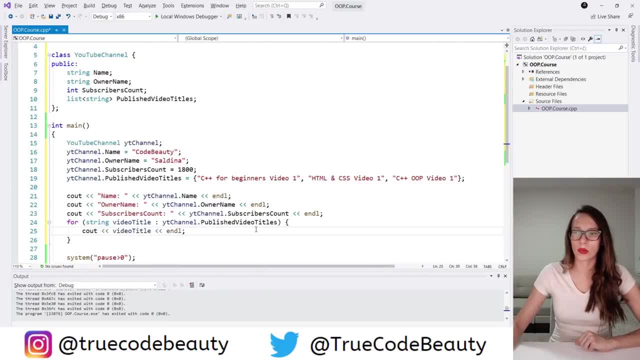 And I'm going to add an end line at the end as well. And one more thing that I want to write out before: this list is going to be just cout videos Like this: OK, and let's add end line at the end so that it is formatted nicely.